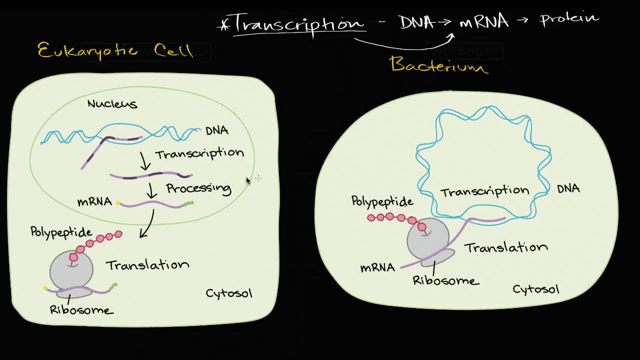 into into an actual protein. But these diagrams give a little bit of an overview of it. It's a little bit simpler in bacteria. You have the DNA just floating around in the cytosol And so the transcription takes place. You start with that DNA. 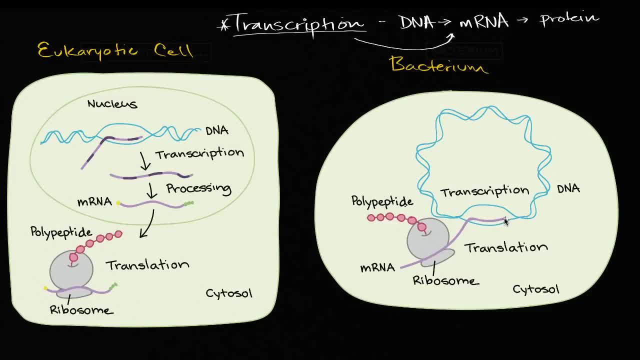 that protein-coding gene in the DNA And then from that you code the messenger RNA. You see that in that purple color right over here- And then that messenger RNA can be involved with the ribosome and that's the translation process to actually produce the polypeptide. 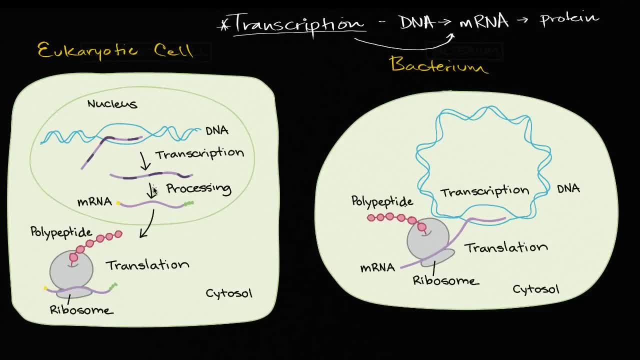 to produce the protein In eukaryotic cells and we're going to get into a little bit more depth in this video: the transcription, the DNA to mRNA that happens inside of the nucleus, And there's essentially two steps here. 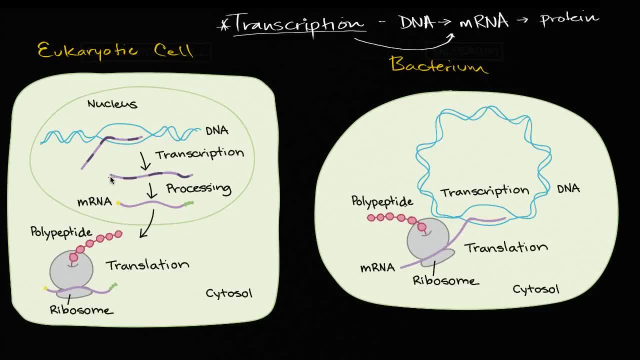 You go from DNA to what we would call pre-mRNA- Let me write that down: Pre-mRNA, which would be, which is depicted right over there, And then it needs to be processed to turn into what we would call mRNA, which then can leave the nucleus. 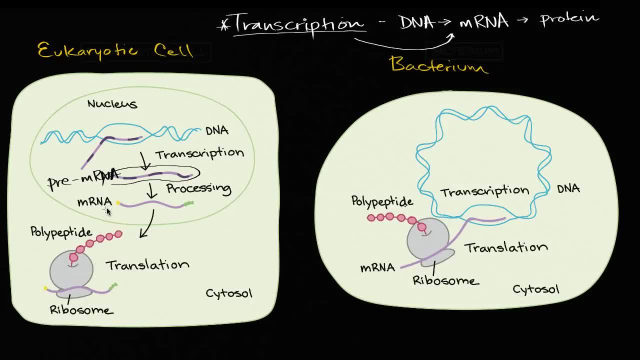 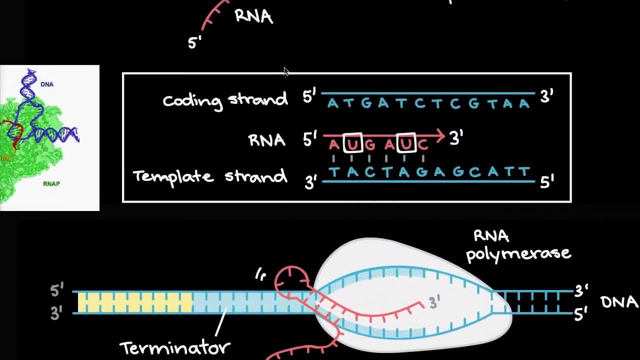 to be translated into a protein. So now that we have that overview, let's dig a little bit deeper into this and understand the different actors and understand if we're talking about a eukaryotic cell. what type of processing might actually go on? 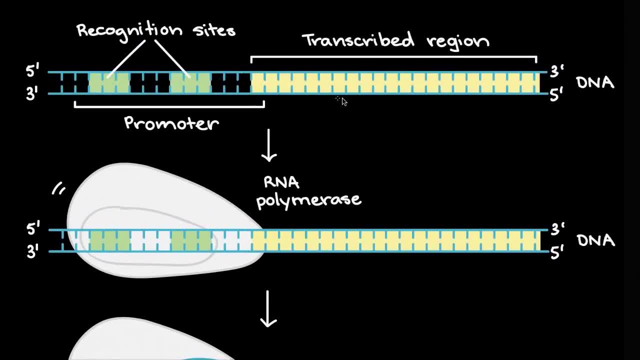 So, right over here we are going to start with the protein-coding gene inside of the DNA, right over here And we are going to the primary protein, which is the DNA, the primary actor. that's not the DNA or the mRNA here. 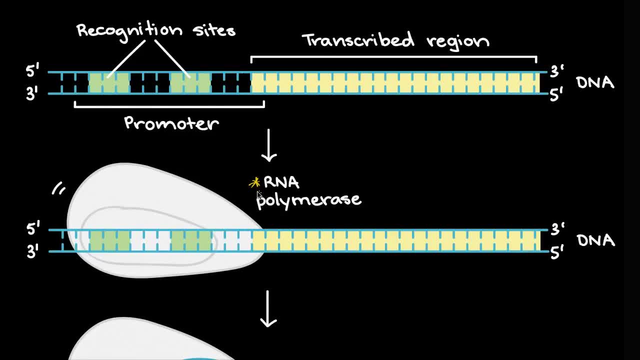 is going to be RNA polymerase. It's used to create a sequence that will become a nucleotide sequence, that will become the messenger RNA. So this RNA polymerase, it needs to know where to start, And the way it knows where to start is it attaches. 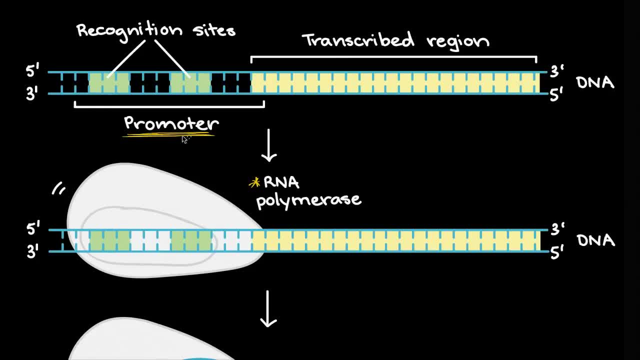 to a sequence of the DNA known as a promoter, And every gene is going to have a promoter associated with it, especially if we're talking about eukaryotic cells. Sometimes you might have a promoter associated with a collection of genes as well. 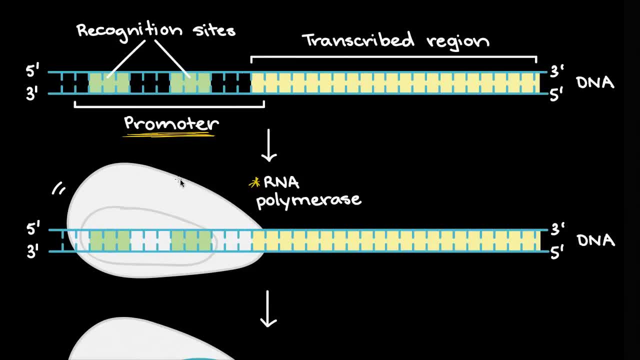 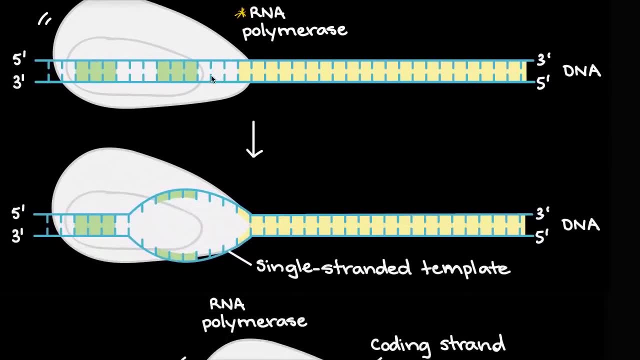 But in general, if you've got a gene, you're going to have a promoter, And so that's where the that's how the RNA polymerase knows to attach right over there, And so once it attaches well, then it is able to separate the strands. 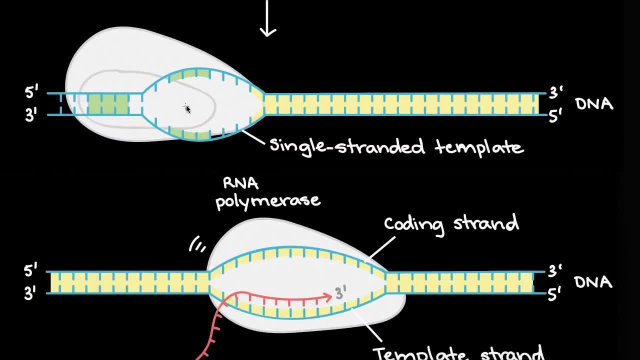 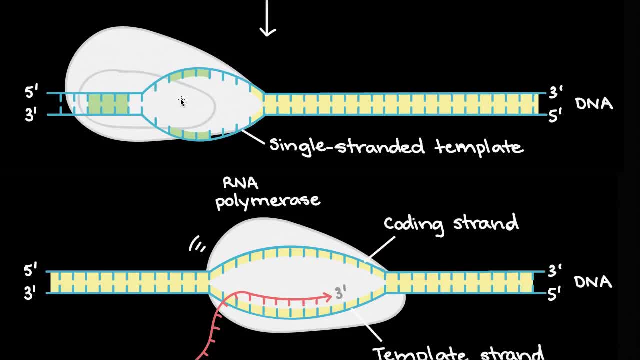 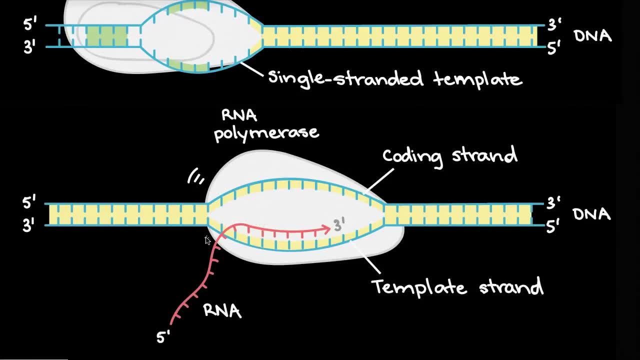 you saw all of these actors, the helicase and whatever else, but this RNA polymerase complex is actually quite capable. Not only it separates the strands and then it's actually able to code for the RNA, And it does that the same way. 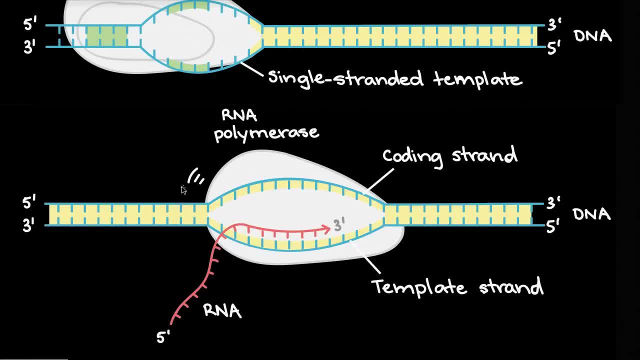 that when we study DNA polymerase, it does it in only one direction. It can only add more nucleotides on the three prime ends. So it encodes from the five prime to the three prime direction. Notice this arrow. here we're extending it. 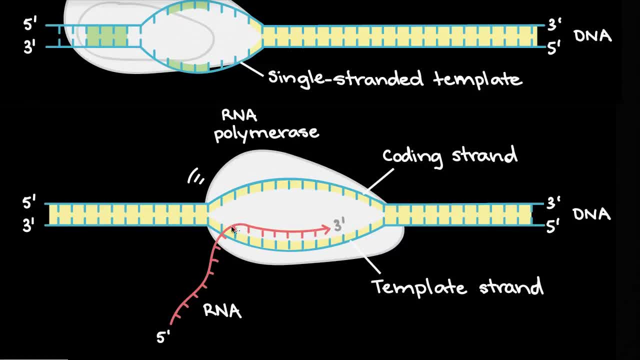 on the three prime end of the RNA, And so, as you can see here, when it does this, it's only encoding one side of, or it's only interacting, I guess you could say- or coding complementary information to one side. But let's think about this a little bit. 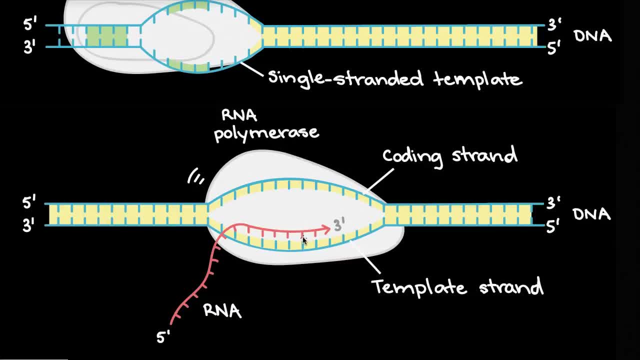 We could call the side that it is forming, that it is interacting with. you could call that the template strand, because that's forming, that's acting. that side of the DNA is acting as the template for forming that RNA. But if you think about the information that that RNA 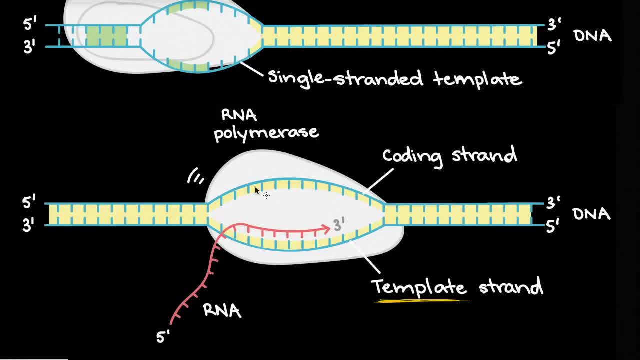 is actually going to encode. well, it's going to contain the same information as the coding strand of DNA, as the other strand of DNA, Because these nucleotides right over here, this nucleotide, it's going to be complementary to this one over here, just as this nucleotide. 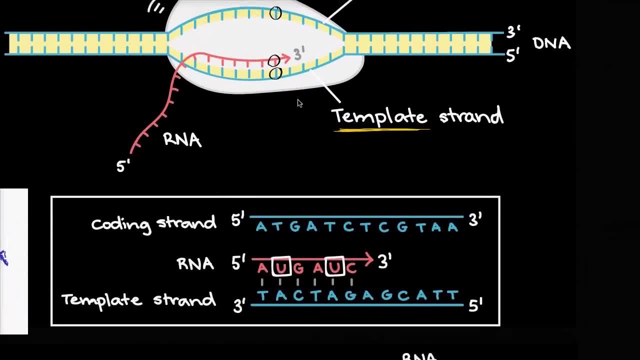 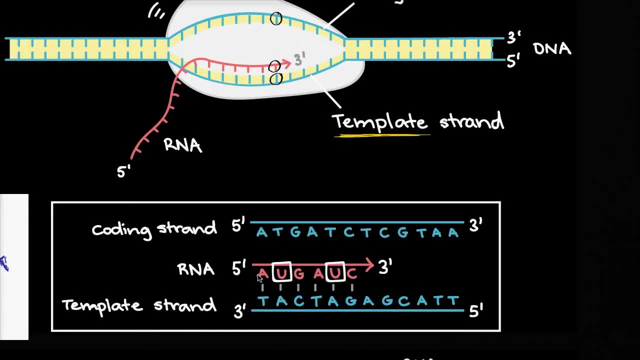 was complementary to that one over there And you can see it in a little bit more depth if we actually were to add the nucleotides. So this is the template strand. If you have a thymine, well, on the RNA. 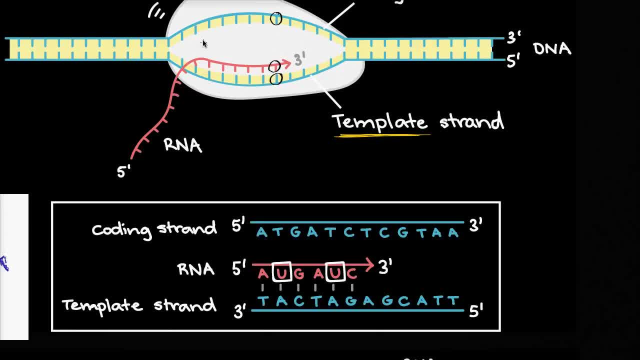 you would have the adenine And look on the coding strand of DNA- the one up here- you would also have an adenine And they are essentially the coding strand and the RNA essentially end up being the same sequence with the one difference is that you won't find. 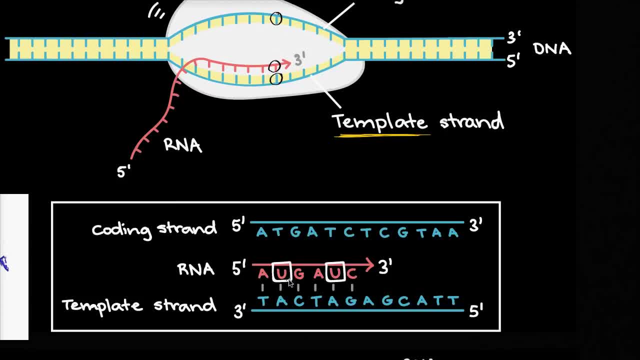 the thymine in the RNA. Instead, you'll find a similar. you'll find a similar nitrogenous base, and that is uracil, But uracil plays the role of thymine, so you're essentially coding the same information. 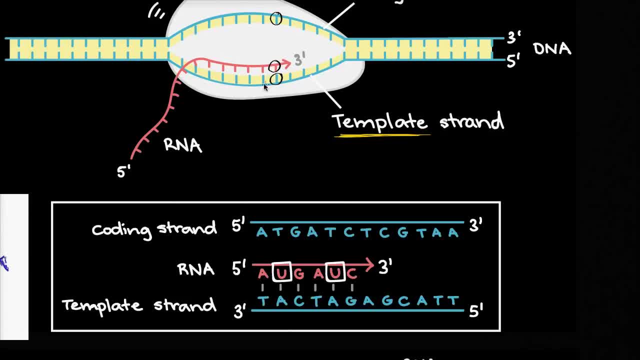 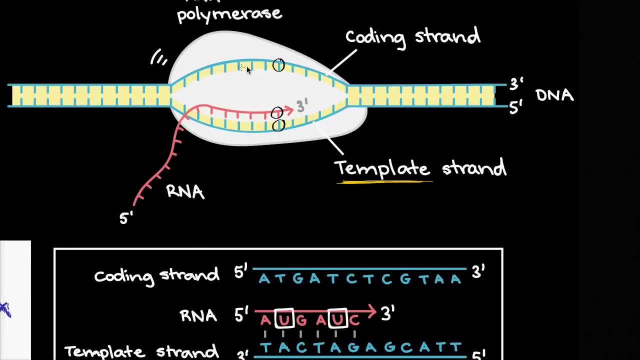 So, once again, this bottom strand is acting as a template, but it's going to be the resulting RNA that gets coded, is essentially going to have the same information that we had in the coding strand. And just to get an appreciation for what this looks like: 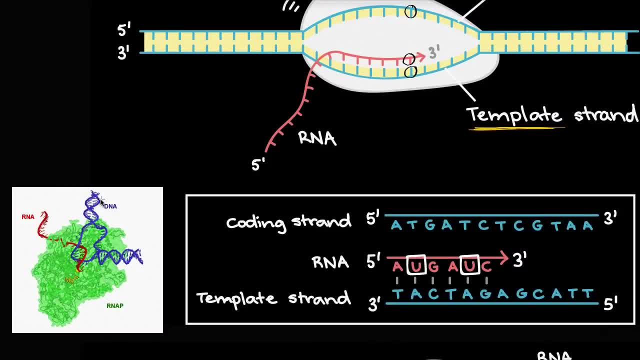 and I would even write, I'd put looks in quotations. I even did little quote things with my fingers when I said that is that it's hard to really visualize what these things look like. but you can see here that the RNA polymerase complex. 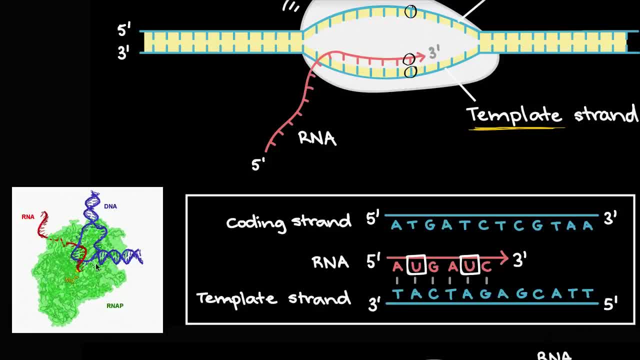 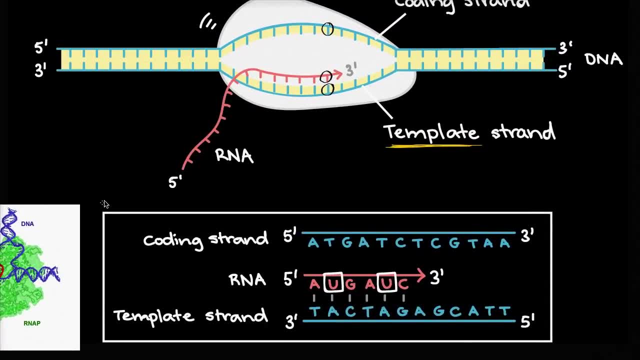 and this is for a specific organism- can be very, very complex and involved, and it's fascinating how these things interact And you know every time you're studying biology and someone like me is going to give you these nice, clean narratives of how these enzymes 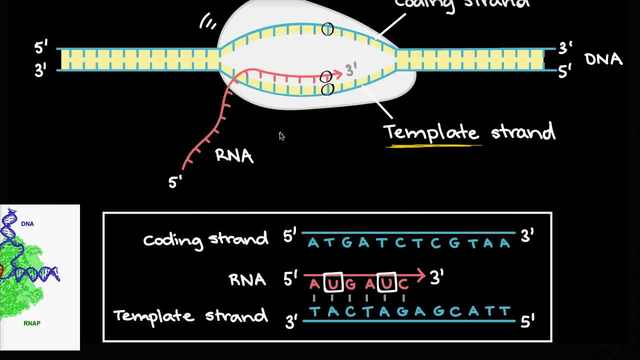 interact with the different macromolecules, like the DNA or the RNA. you should always remember. this is amazing. These are these molecules interacting with each other, bouncing into each other. It's happening incredibly fast inside of the cell. You should be in awe of this. 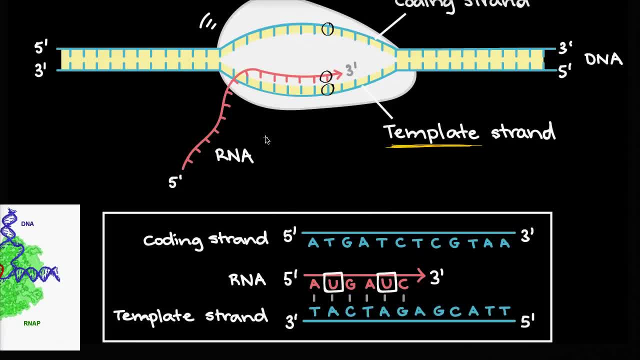 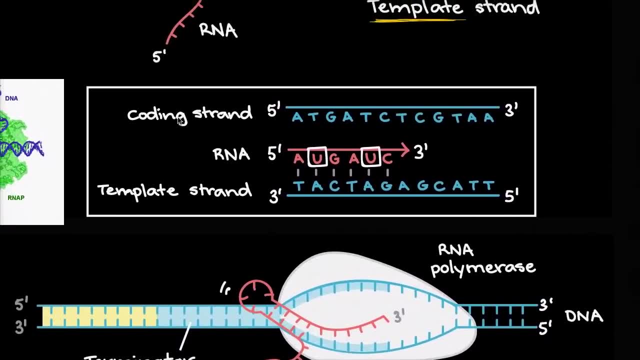 It's happening in all of your cells, or as we, as we speak. so this is pretty incredible stuff. So the next thing you have to think about: you know this: right over here, we are extending the RNA. Well, when does this thing actually stop? 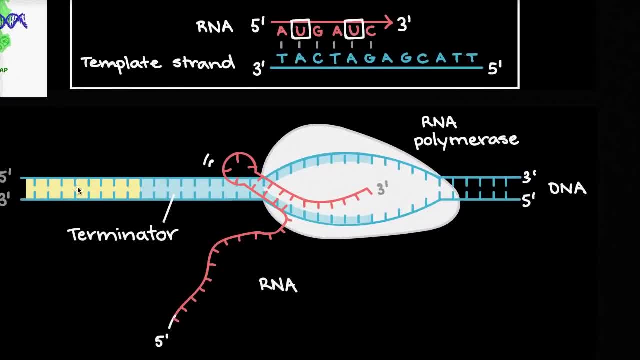 And it stops once we so this RNA polymerase is gonna keep going on. and then this blue where we've labeled this a terminator. So let me write: so this area is a terminator and there's multiple ways that that signals to the RNA polymerase that hey, it's time to stop. 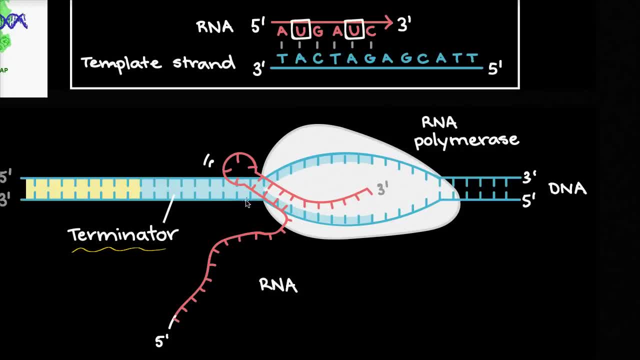 Or, and more particularly, that it somehow creates something structurally that the polymerase just lets go. One mechanism that's depicted right over here is that the mRNA that's coded- and this is typical or this can happen in bacteria- is that the mRNA that's coded forms a hairpin. 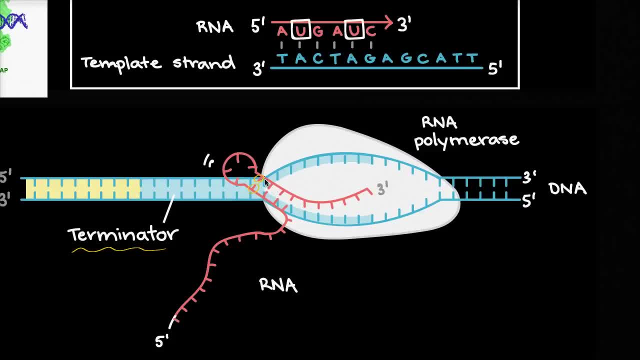 So it has to have the right complementary base pairs, base pairs right over here. It has to form this hairpin, but this hairpin, along with the things around the hairpin, essentially make it impair the polymerase to keep on going. 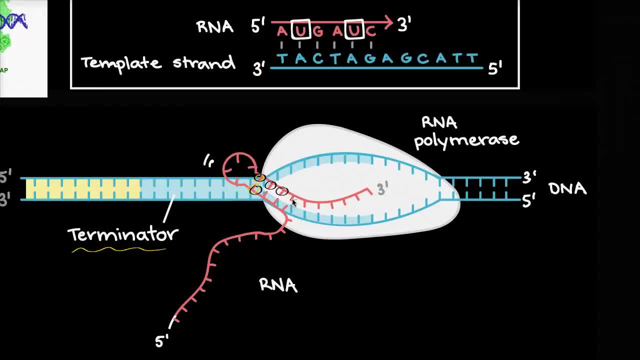 and so the complex kind of changes a little bit, and so it lets go, or at least that's how people believe it. There's other forms of how the terminator can act. It might be sequences that parts of the polymerase complex recognize. 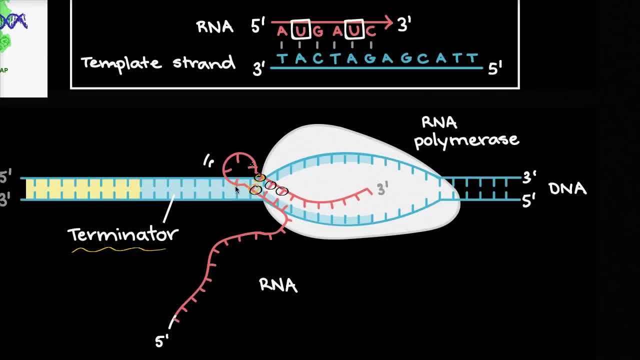 and it forms, it makes a conformation change so that the RNA polymerase lets go. Now, if we're talking about it, if we're talking about a prokaryote, we're done. We would have formed, this would be our messenger RNA. 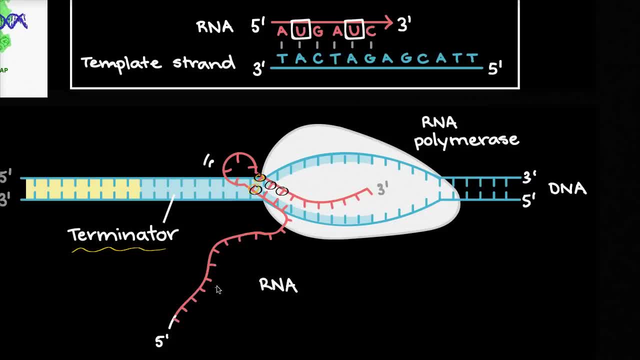 which then can go to a ribosome and then be translated into a protein. but if we're talking about a eukaryote, well then we have to do a little bit of processing If we're talking about a eukaryote. 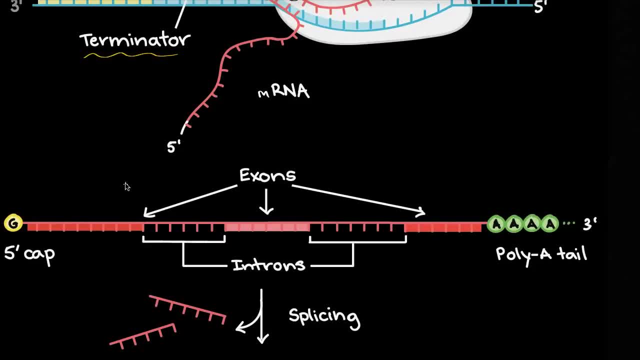 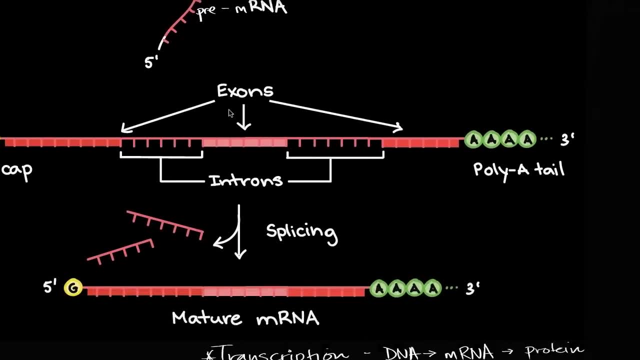 if this is a prokaryote right over here, this would be our mRNA. If this is a eukaryote, then this is our pre-mRNA, which now has to be processed. and you might say: well, how is that going to be processed? 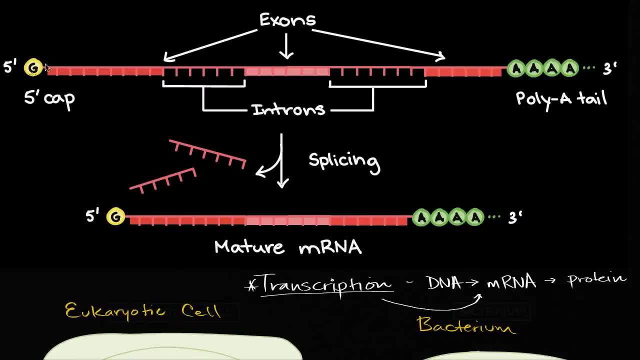 Well, there's a couple of things that are going to be done. Some things are going to be added at the beginning and the end of the mRNA, the five prime cap. This is a modified guanine- modified modified guanine right over here. 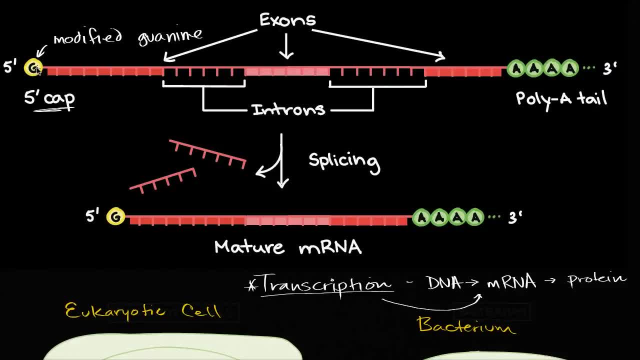 which is going to help in the translation process as the ribosomes attach onto it. And then you have this poly-A tail- and it's called a poly-A tail because it has a bunch of adenines at the end, right over here. And these not only help in the translation process. 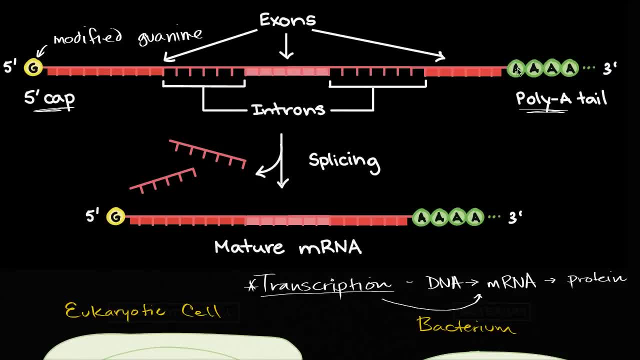 it helps make sure that the information is more robust, that the ends of the mRNA don't in some way become, or makes it less likely that they're going to become, damaged. Now the other thing that needs to be processed, and this is one of those fascinating things. 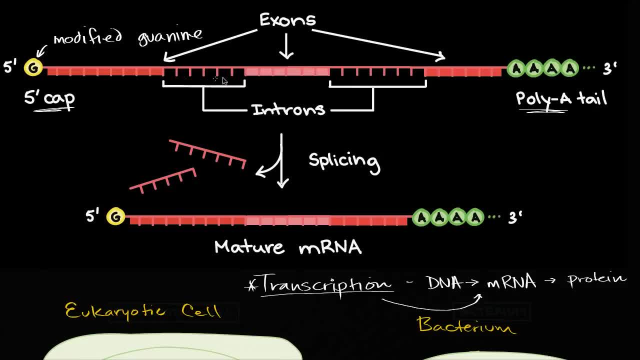 in evolutionary biology is that we will have. in this mRNA sequence. you're going to have parts of the sequence which we currently consider to be nonsense, sequence, nonsense sequences and we call them introns, And I'm going to put it in quotes: